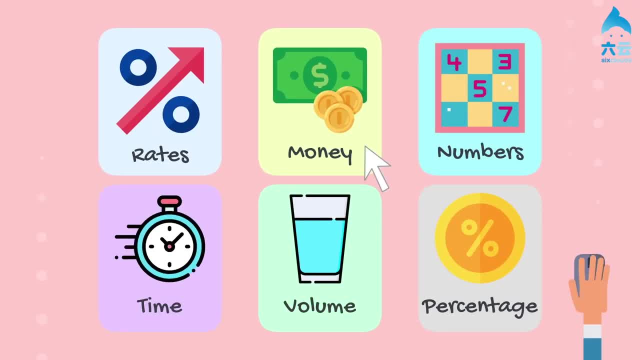 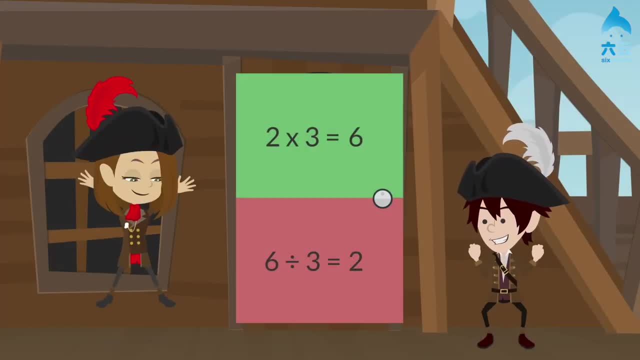 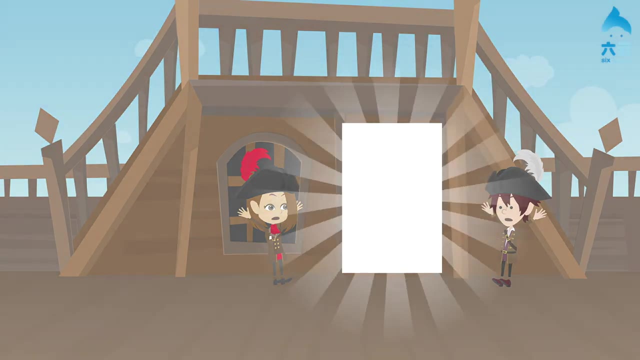 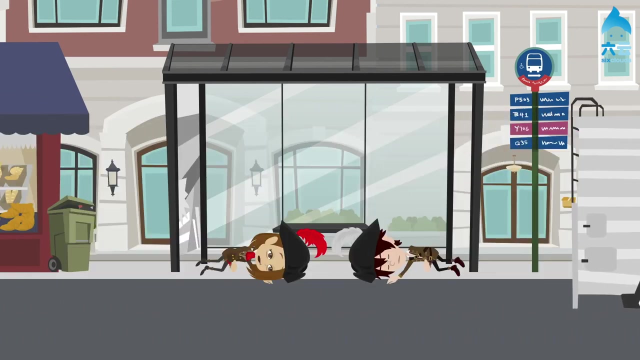 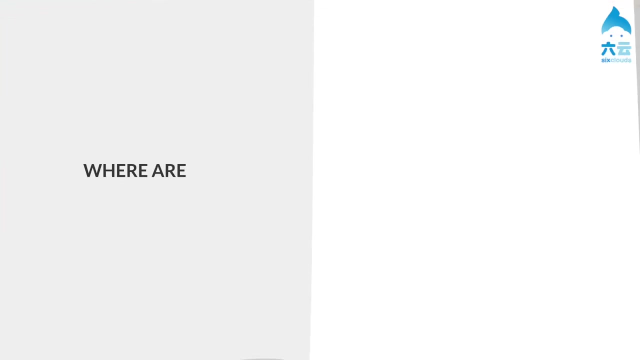 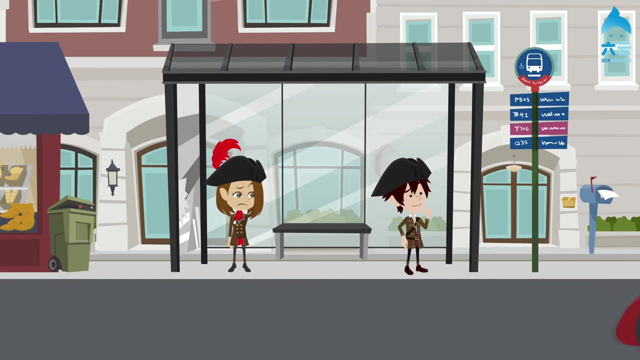 Where are we? I don't know. We are in the future. What are all these strange moving things? And they carry people. Let's get on one of them. Hey, you need to pay 50 cents to get on the bus. 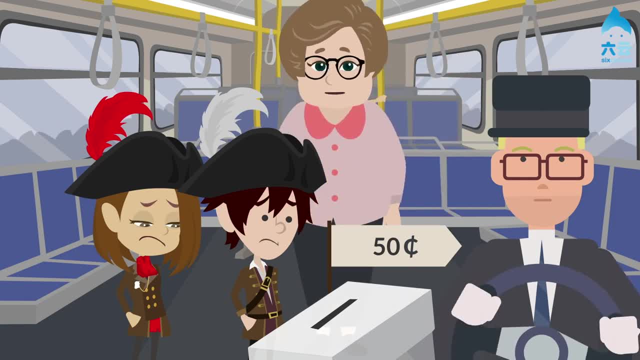 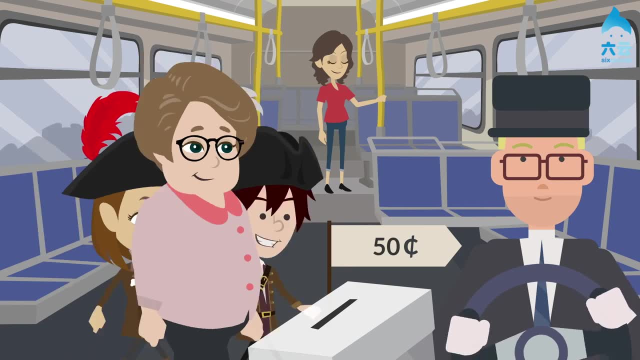 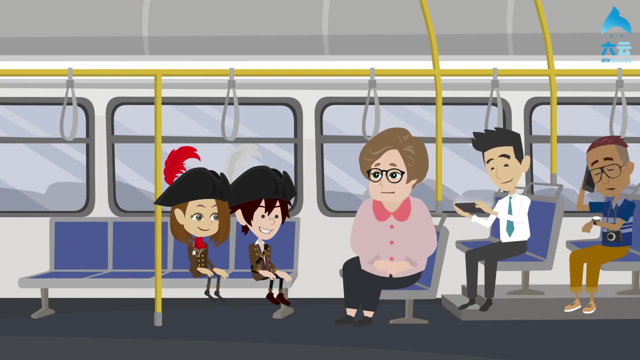 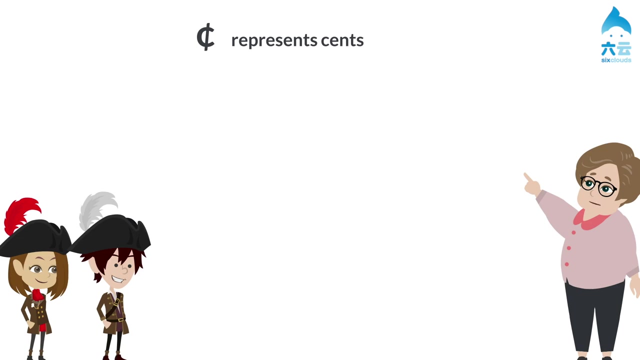 You seem to be from elsewhere. I'll pay for them. Where are you from? City of Water, Interesting name. Thank you, madam, for paying for us. Madam, what does this symbol mean? This symbol represents cents. This is a one-cent coin. 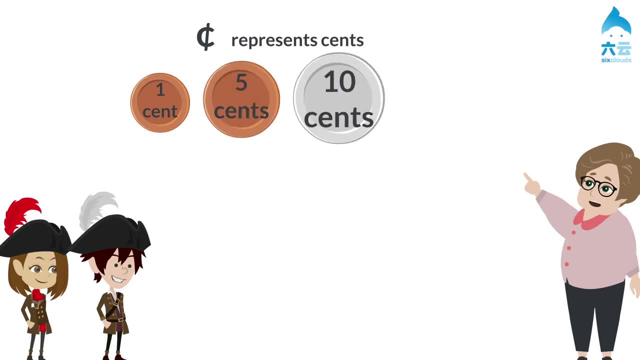 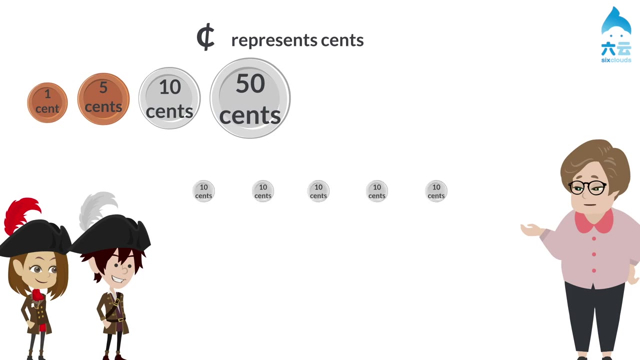 Five-cent coin. Ten-cent coin. Fifty-cent coin. Oh, so does that mean we can use this fifty-cent coin to pay for the bus ride just now? Yes, We can also use five ten-cent coins to pay. The amount is the same as one fifty-cent coin. 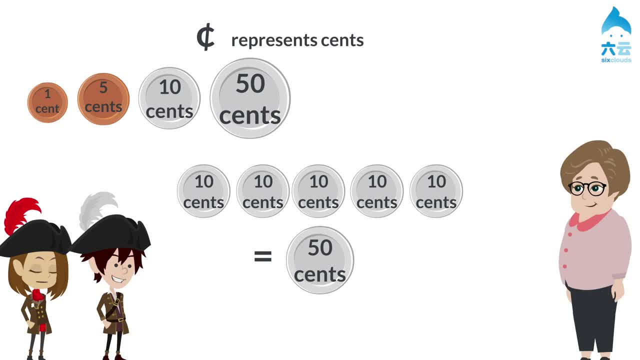 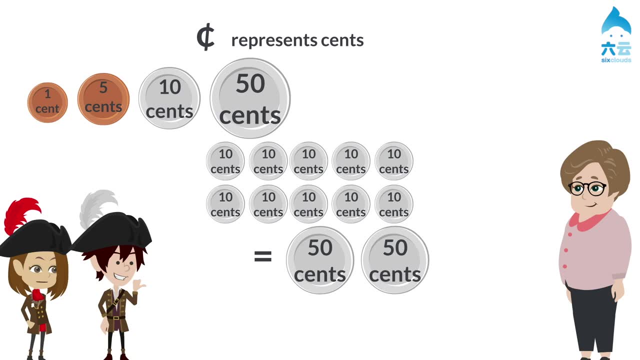 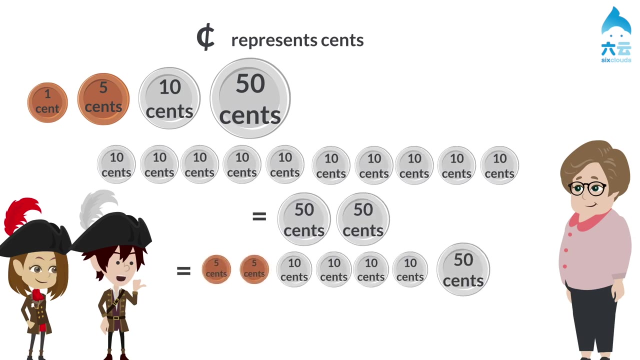 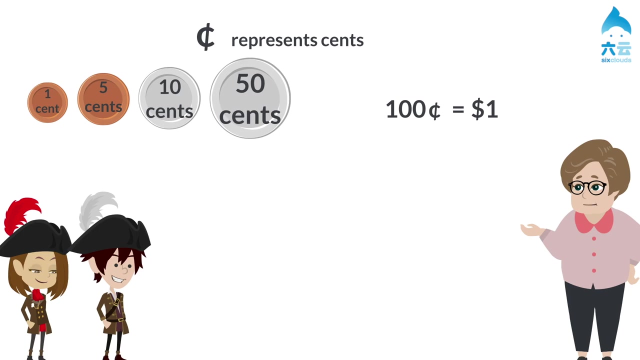 The fee for David and me will be one hundred cents. That means we can pay with ten ten-cent coins or two fifty-cent coins, Or we can pay two five-cents, four ten-cents and one fifty-cent coins. One hundred cents is equal to one dollar.